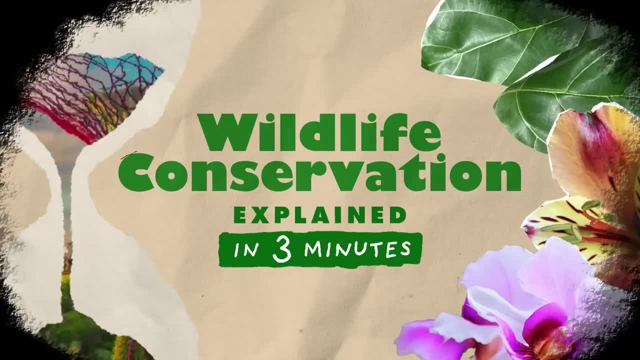 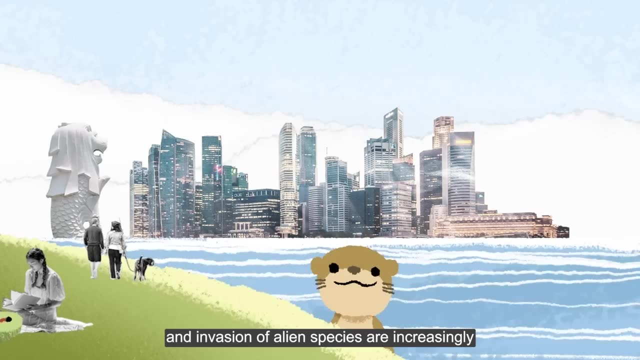 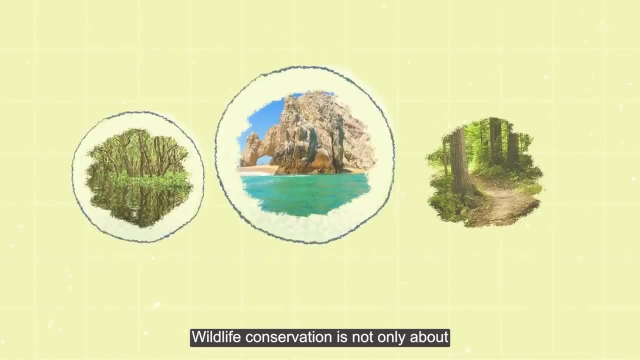 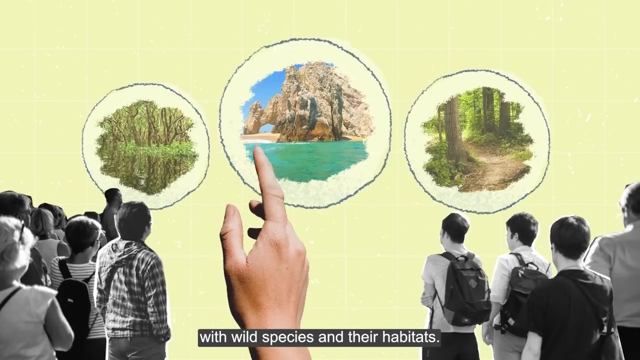 Urbanization, climate change, illegal wildlife trade and the invasion of alien species are increasingly threatening the lifespan of wildlife species. Wildlife conservation is not only about the survival of plants and animal species, but also educating people on living harmoniously with wild species and their habitats. 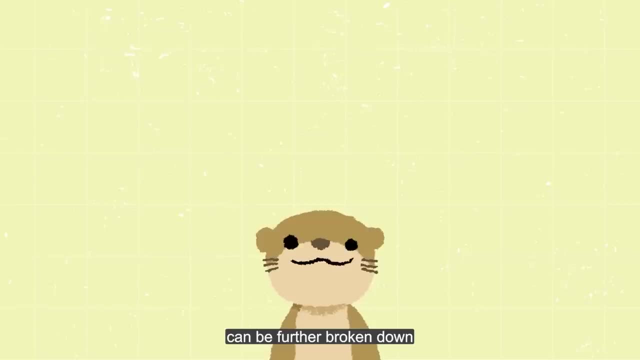 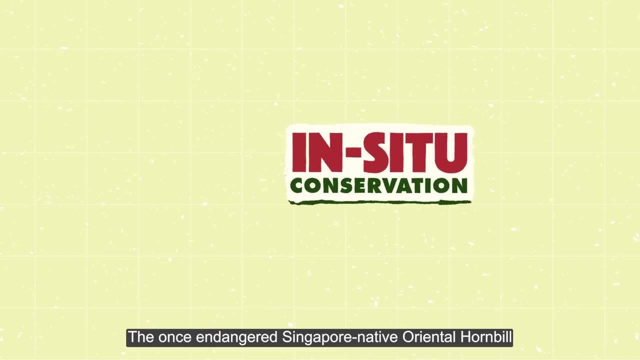 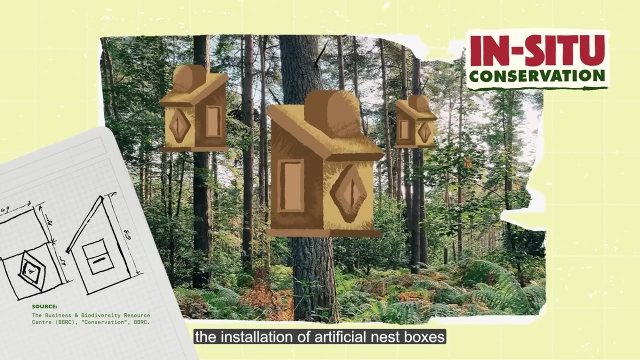 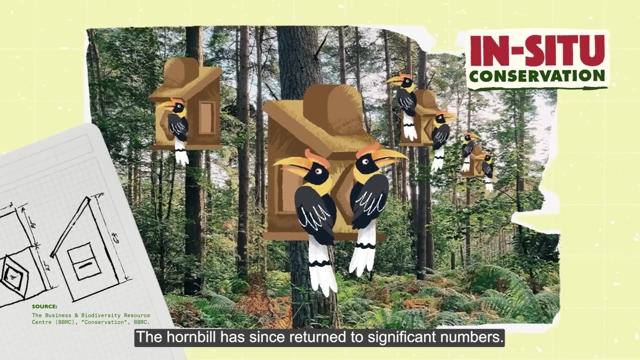 Wildlife conservation can be further broken down into in-situ and ex-situ conservation. The once endangered Singapore native oriental hornbill saw hope with a Singapore hornbill project. The installation of artificial nest boxes provided a safe environment for breeding. The hornbill has since returned to significant numbers. 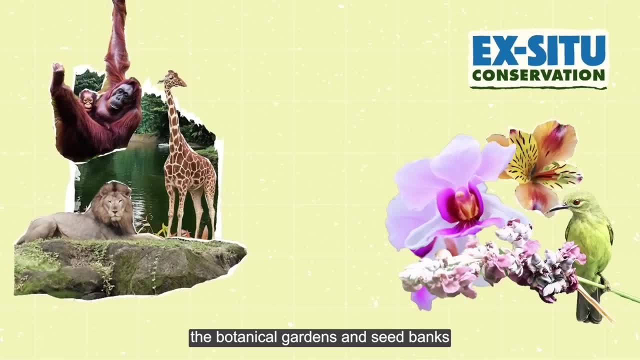 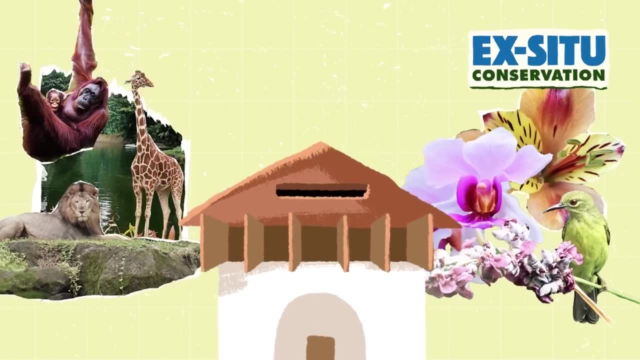 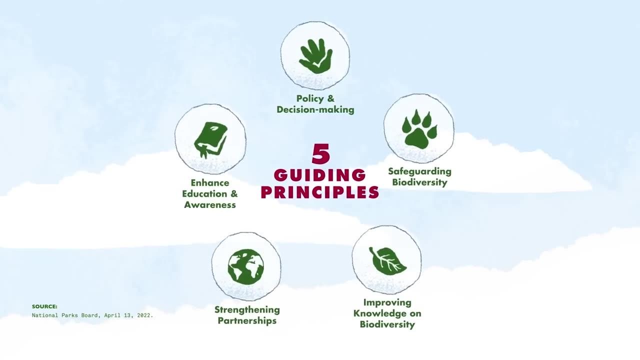 In Singapore, places such as our zoo, the botanical gardens and seed banks protect local wildlife outside of their natural habitats. Did you know that Singapore has five guiding principles to support wildlife conservation? For wildlife to thrive in Singapore, safeguarding our biodiversity is fundamental. 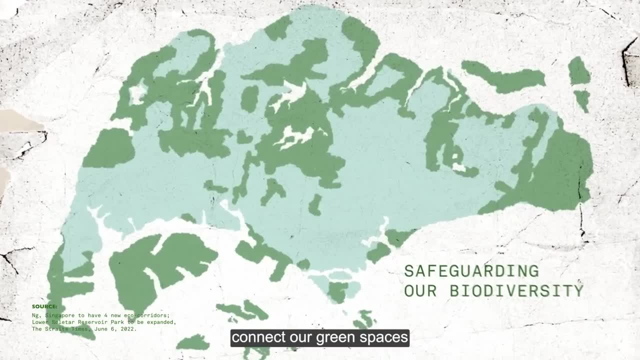 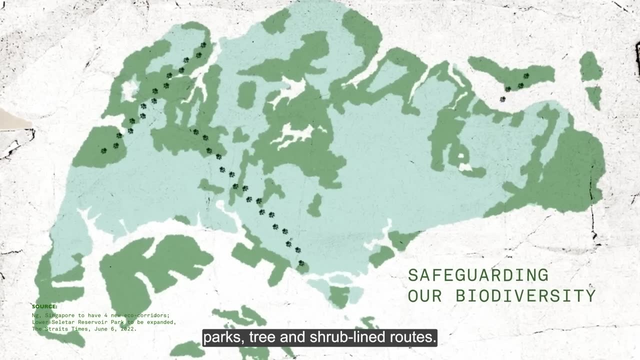 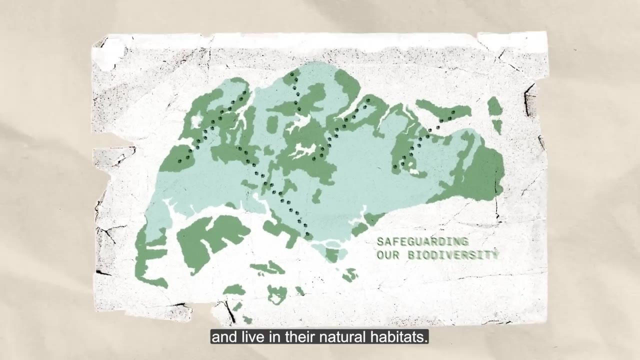 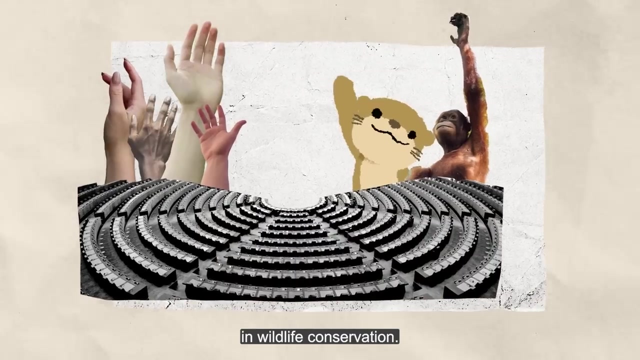 Singapore's nature corridors connect our green spaces for wildlife to thrive in forested patches, parks, tree and shrub-lined routes. These corridors act as a safe highway for wildlife to intermingle and live in their natural habitats. Singapore also recognises the importance of policy in wildlife conservation. 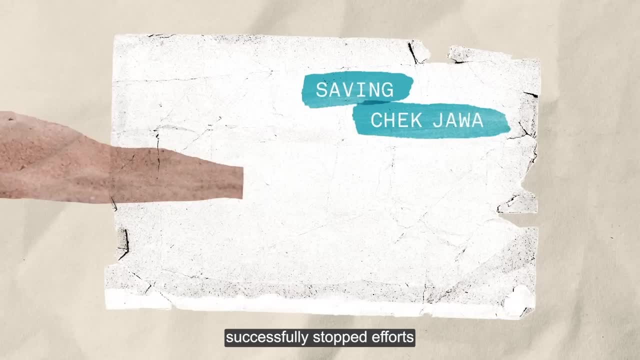 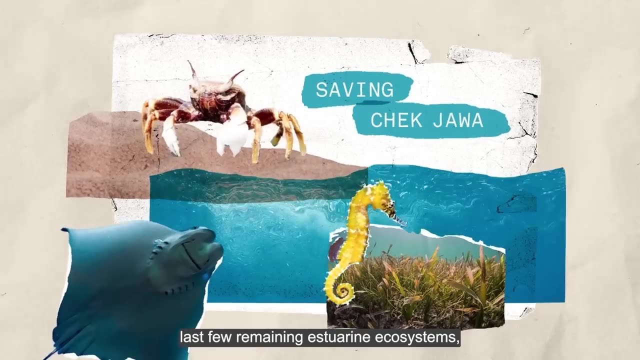 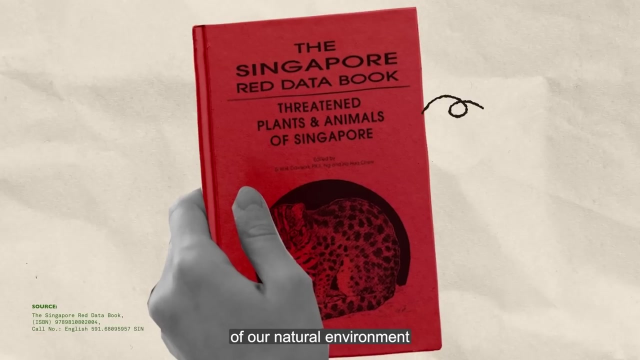 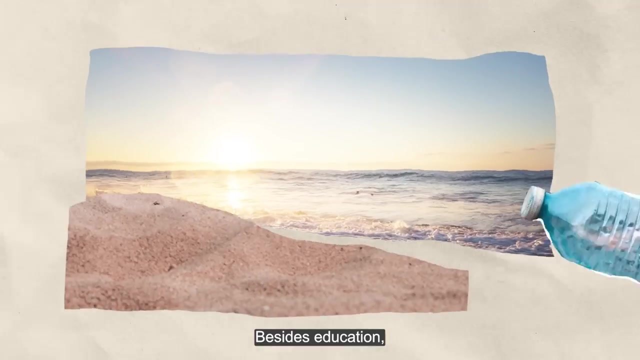 The Saving Chick Jawa initiative successfully stopped efforts on land reclamation over one of Singapore's last few remaining estuarine ecosystems, which are home to diverse species. The continued study of our natural environment also plays a pivotal role in wildlife conservation. Besides education, promoting volunteerism in conservation efforts bolsters protection of Singapore's wildlife. 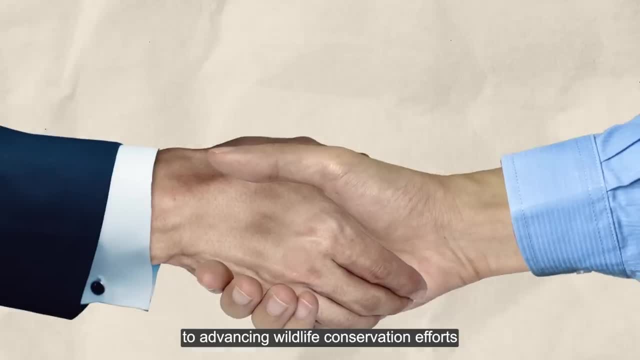 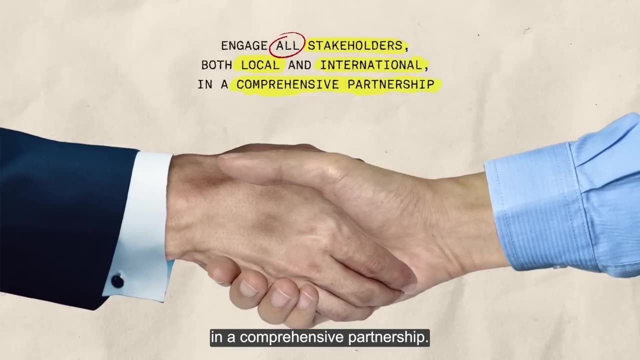 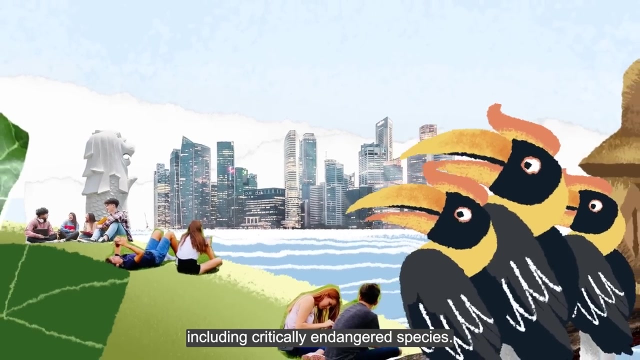 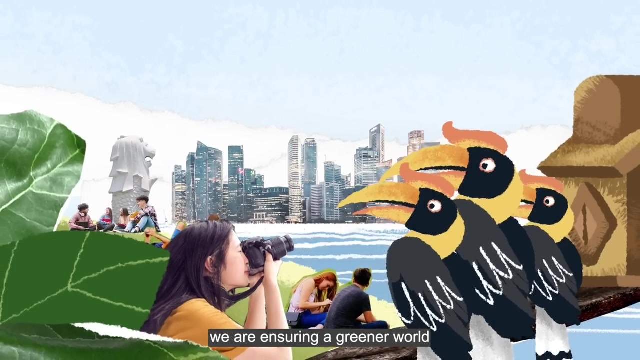 The final key to advancing wildlife conservation efforts is to engage all stakeholders, both local and international, in a comprehensive process. Singapore is home to diverse wildlife, including critically endangered species. By protecting our natural heritage and ecosystems, we are ensuring a greener world for our future generations.